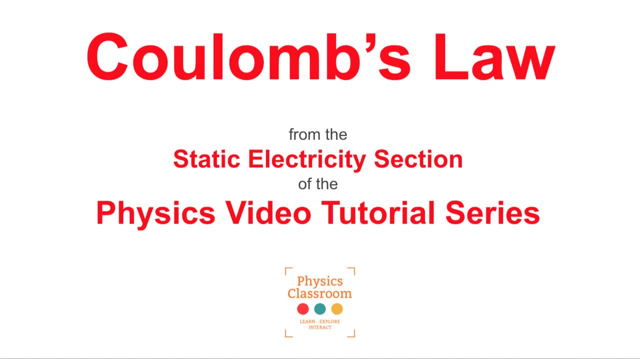 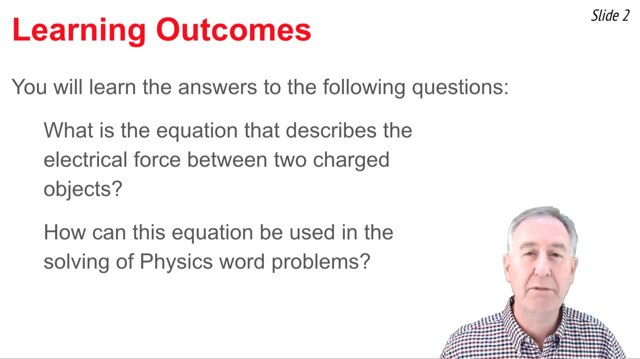 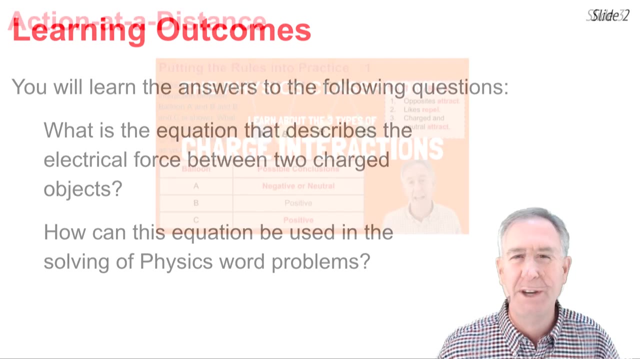 Welcome to the physics classroom's video tutorial on static electricity. The topic of this video is Coulomb's law, and here's what we wish to learn today: What's the equation that describes the electric force between two charged objects, and how can we use this equation to solve physics word problems? I'm Mr H. Let's get started In a previous video. 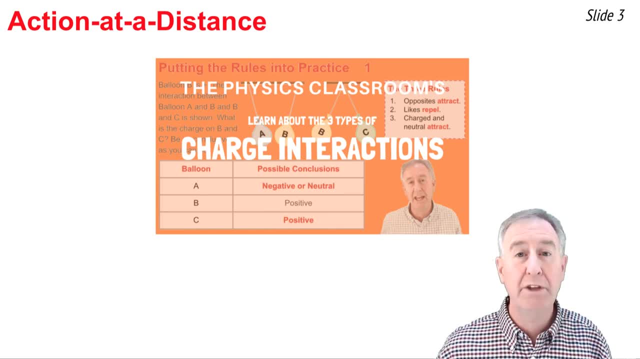 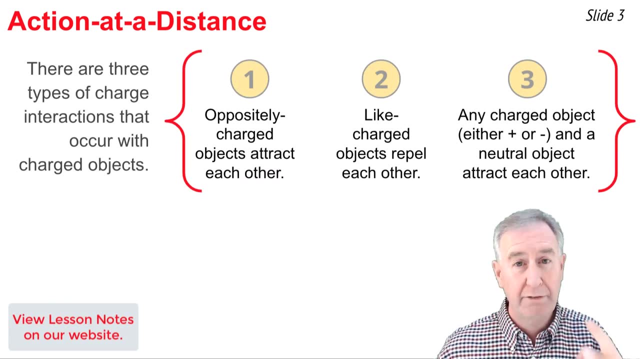 this one I discussed charge interactions. If you need to review, you'll find a link to it in the description section below. We discussed three types of charge interactions in that video. First, oppositely charged objects will attract one another. Second, like-charged objects will. 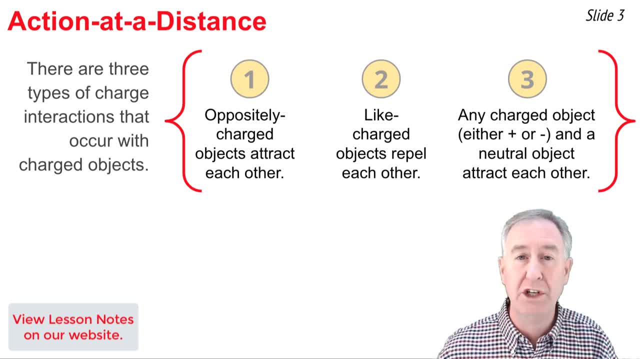 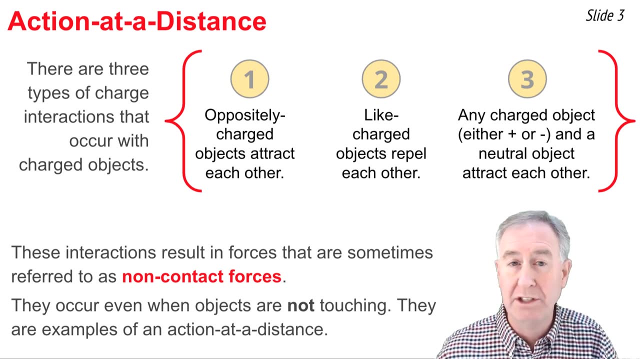 repel one another. And third, any neutral and charged object will interact so as to attract one another as well. These three interactions result in forces that we call non-contact forces, because they occur even when the two objects are not touching one another over some distance of severity. 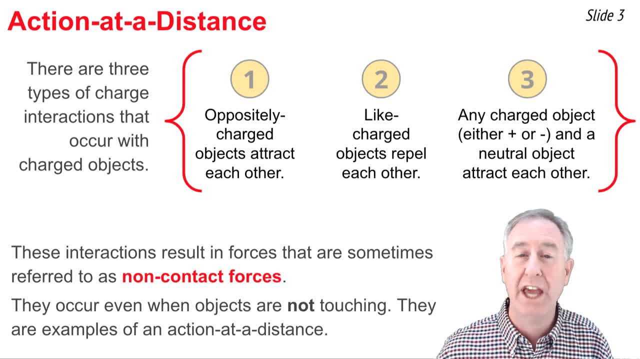 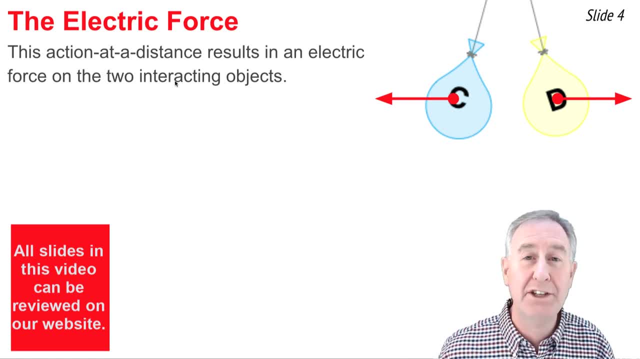 separation. We sometimes refer to them as actions at a distance. These hanging balloons provide examples of an action at a distance. An action at a distance always results in two forces, one on each of the interacting objects. We call these forces electric forces and, like any force, they're subject to all the 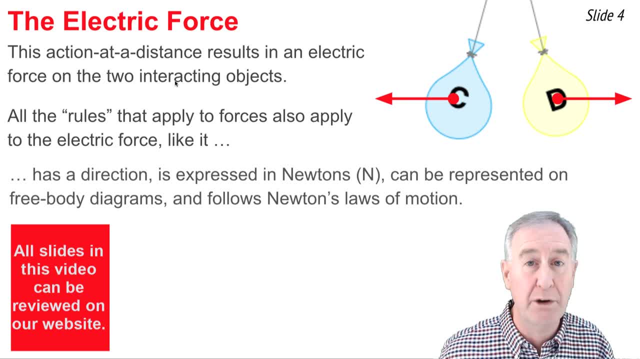 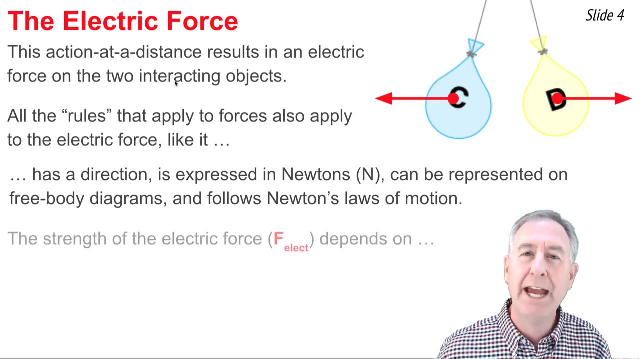 rules that apply to forces, like the idea that they're vectors and they have a magnitude and direction. Their magnitude is expressed in units of Newton's, They can be represented on free body diagrams by vector arrows and they're subject to all of Newton's laws of motion. 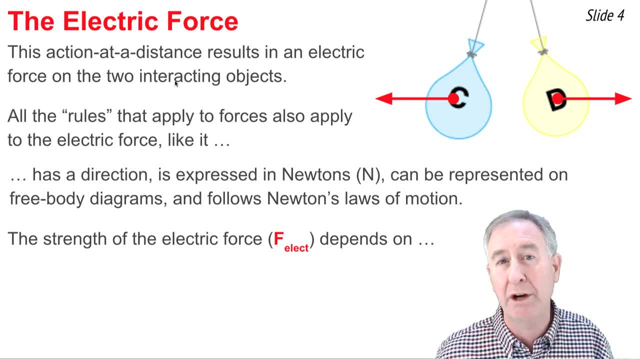 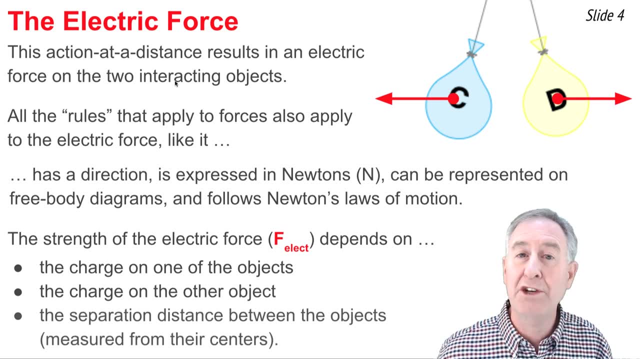 The magnitude of the electric force is dependent upon three variables: the amount of charge on one of the object, the amount of charge on the other object and the separation distance between the two objects. We measure the separation distance not from their nearest edges but from the centers. 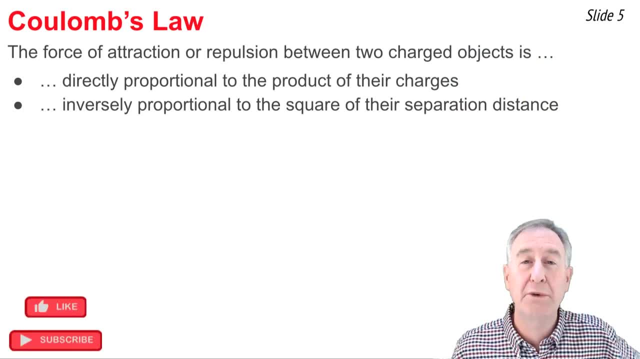 of the two objects. Coulomb's law expresses the relationship between the electric force and the variables that affect it. The law can be stated like this: The electric force between two charged objects is directly proportional to the product of their charges and inversely proportional to the separation distance. 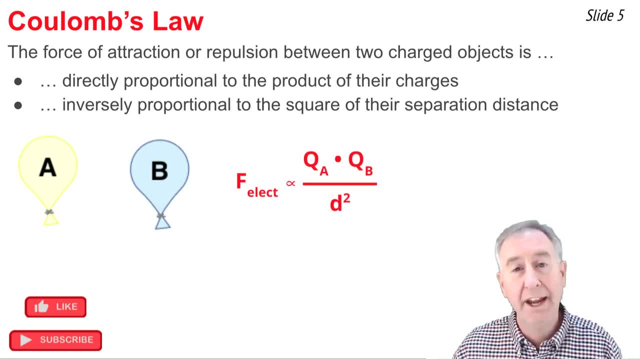 This proportionality statement can be expressed like this: Here, Q represents the quantity of charge on object A and object B and D represents the separation distance. If I wish to express this by an equation, I need to use a proportionality constant. 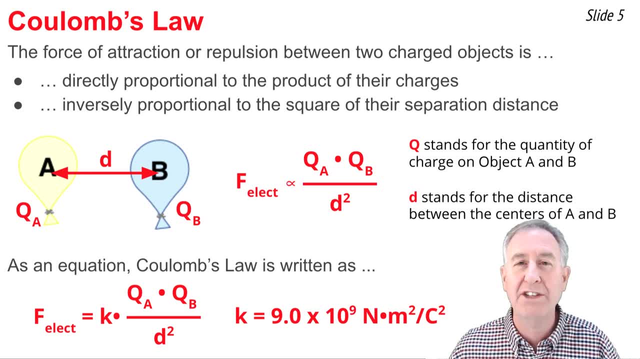 k. It can be written like this: where k is sometimes referred to as the Coulomb's law constant, Its value is 9.0 times 10 to the 9th Newton's times: meter squared per Coulomb squared. Because of these units, when I use this k value to solve for electric force, I have: 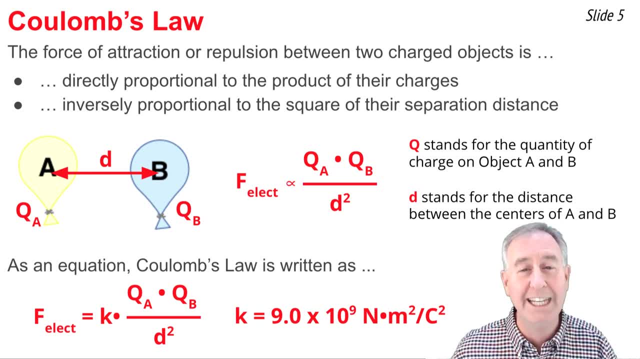 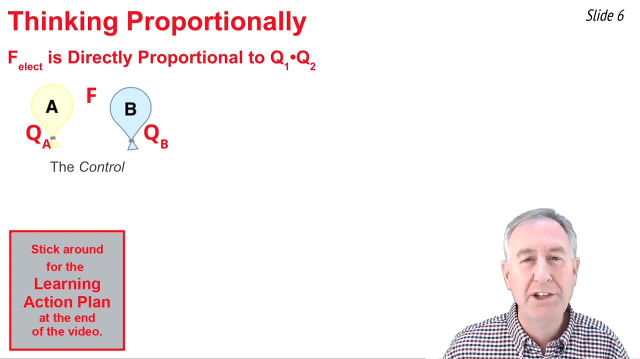 to use q in units. In a physics course, there are typically two ways we use Coulomb's law. One way is to think about how a change in one of the variables would affect the electric force, For instance the change in one of the q values. 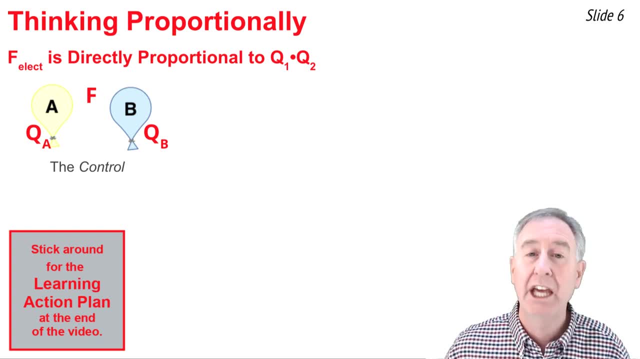 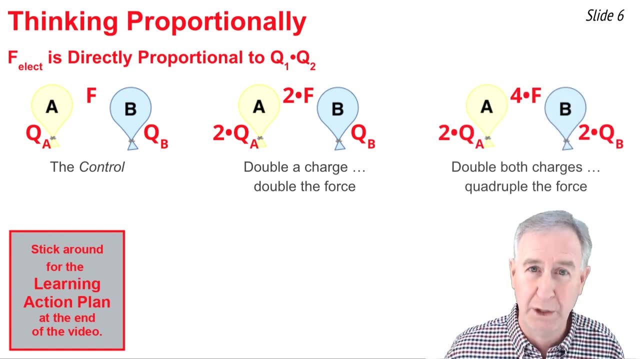 Here we have two balloons with charges qA and qB. If we double one of the charges, that would double the force. If we double both the charges, well, that would quadruple the force. If we double both the charges, well, that would quadruple the force. 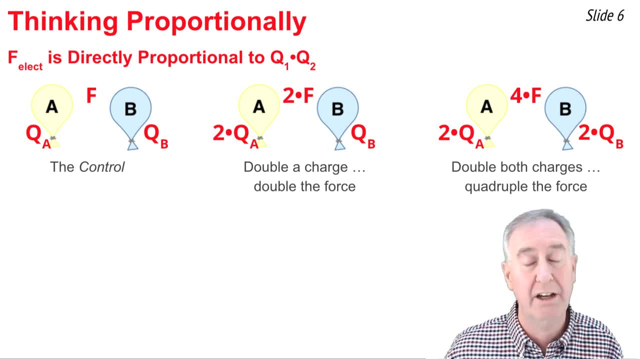 If we double both the charges, well, that would quadruple the force. But- this is a particularly important aspect—the difference in the electric force is directly proportional to the product of the charges, But it's also inversely proportional to the distance of separation squared. 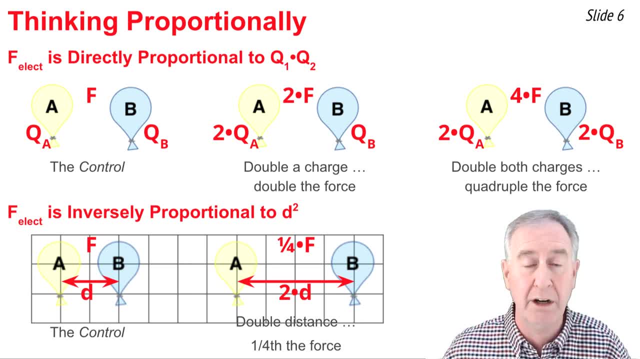 So if we start with two balloons that are two units of distance apart and then we separate them by four units, we've increased the d-value. That should decrease the f-value. In fact, if you double the distance, you should decrease the f-value by 2 squared. 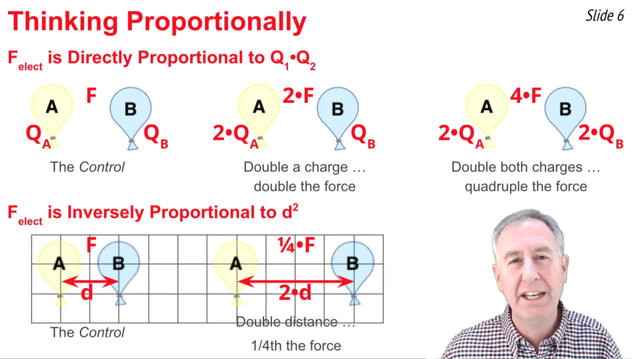 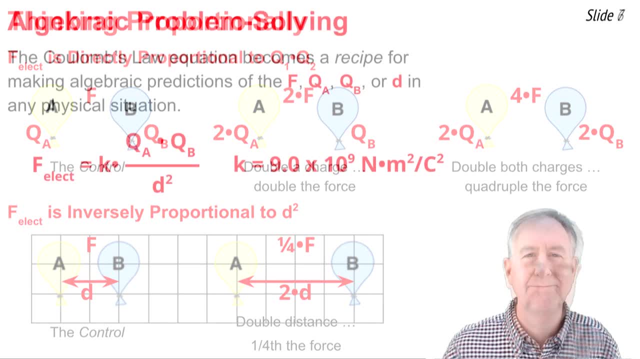 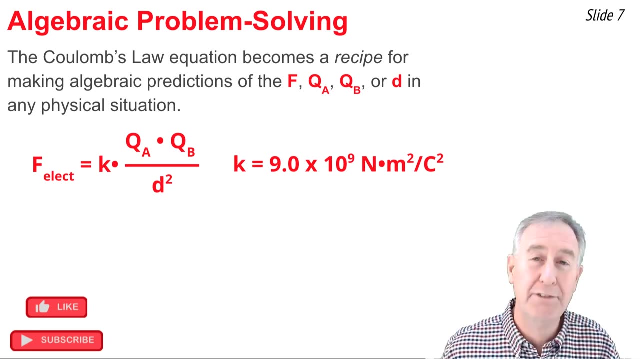 You would then have ¼th of the force. So it's that simple of the force. This idea of thinking proportionally about the equation will be used much more intensely in the next video. The second way that Coulomb's Law is often used is as an algebraic recipe for solving for an unknown in a physics. 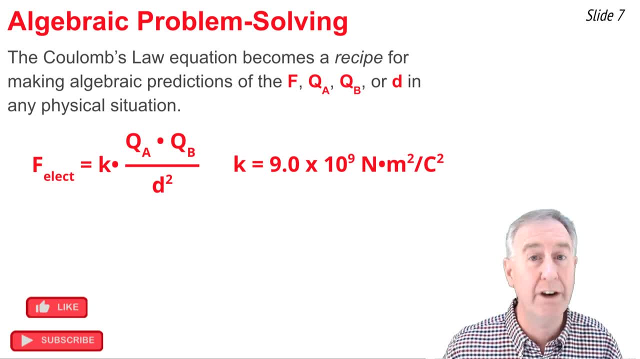 word problem. Here's the equation. You'll note that there are four variables in it. If you know the value of any three, you can solve for the fourth variable. One caution you'll have to take as you solve such problems is that the value of Q is. 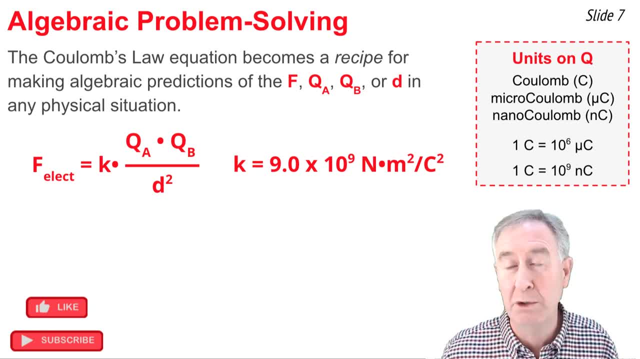 seldom given in units of Coulombs, So you'll have to use the above conversion information in order to convert from other units to Coulombs, For instance, from micro-Coulombs to Coulombs or nano-Coulombs to Coulombs. Here's a: 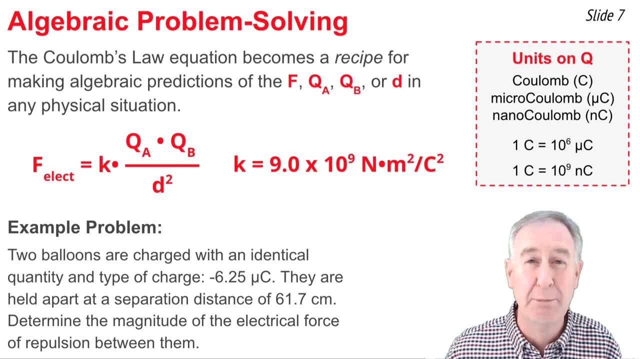 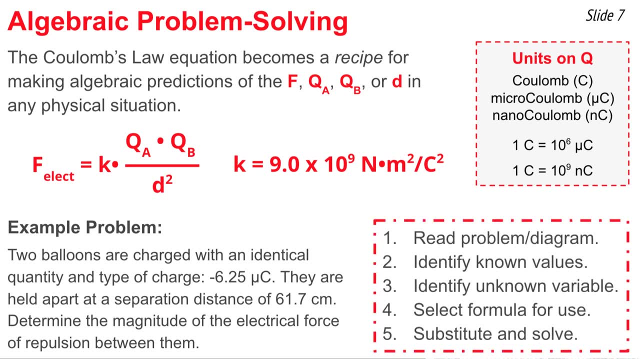 typical problem. In order to solve this problem, or any problem in physics, it's always wise to follow five steps. The first step is to read the problem into diagrams In order to develop a mental picture. The second step is to identify known values. 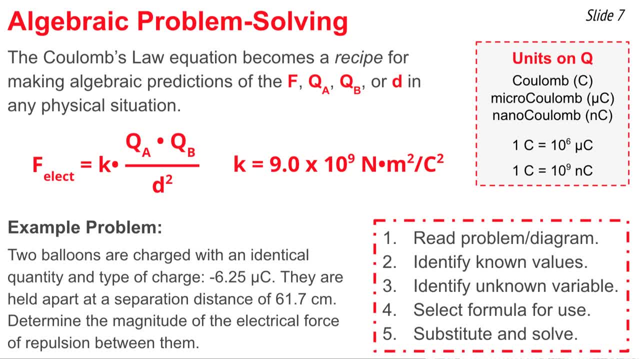 of the variables in the equation. The third step is to identify the unknown variable. You should express these variable values in the unknown using the symbols of the equation. For instance, you might say: QA equal negative six point two, five micro-Coulombs. Then select a formula for use, Maybe even rearrange it. 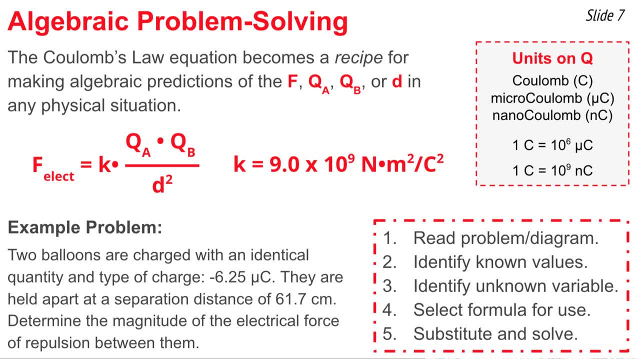 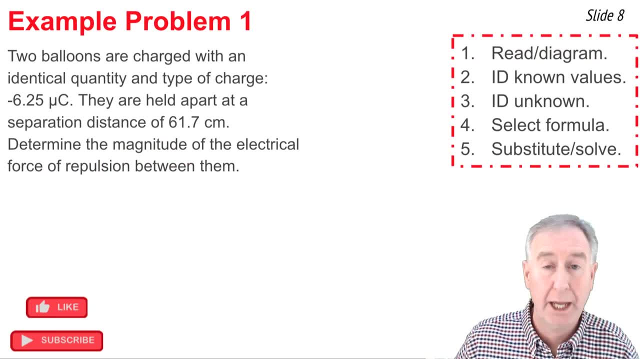 to get the unknown variable by itself. Finally, substitute known values into the equation and solve for the unknown variable. Here's my first example problem. I'm going to read and then diagram the situation: Two balloons are charged with an identical amount of charge of negative. 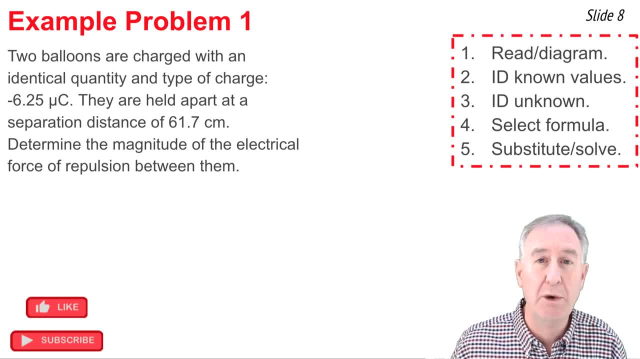 six point two, five micro-Coulombs. They're held a distance of sixty one point seven centimeters apart, Determine the magnitude of the force. So my mental picture is: I have two balloons, I know the QA and QB value of the balloons and the separation. 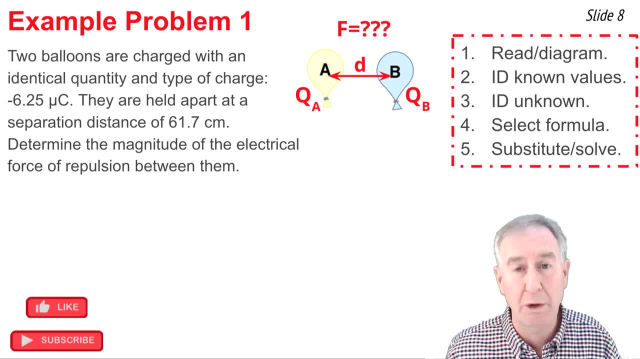 distance. I'm looking for my F electrical. I'm going to record what I know in this problem. I know QA is the same as QB. It states an identical amount of charge. I know the value is negative six point two, five micro-Coulombs. But you'll note I've 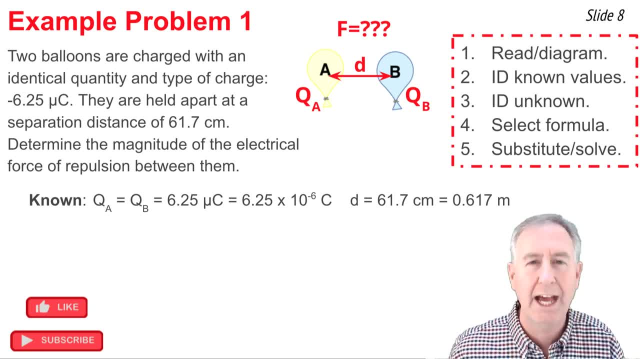 left out the negative, because it only is going to complicate matters. I'm not interested in anything other than the magnitude of this force. Having the sign of the charge isn't going to help me to do that. I also know that D is equal. 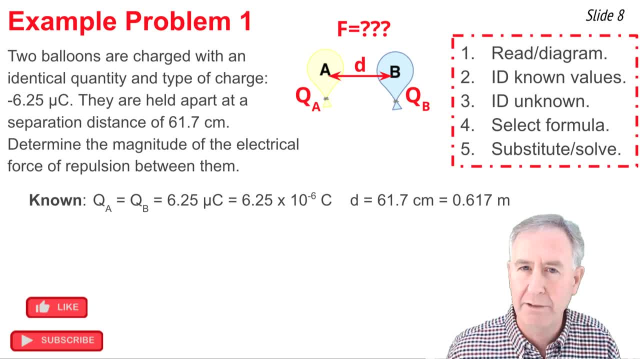 to sixty one point seven centimeters. You'll note that I've done conversions from Coulombs to micro-Coulombs and from centimeters to meters. I'm looking for the F electrical, and here's my equation. I'm ready to go, I write the equation down and then I make. 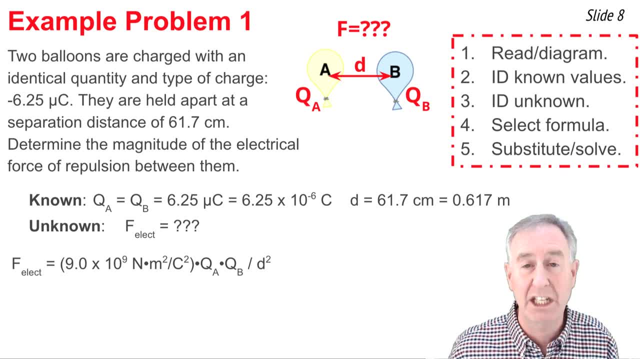 substitutions of QA, QB and D into this equation. I use units of Coulombs and meters because that's the units used on the value of K. Here's my substitutions. Now I pull out my calculator, I write down here the numbers between the F and QAB and what I'm comfortable with. 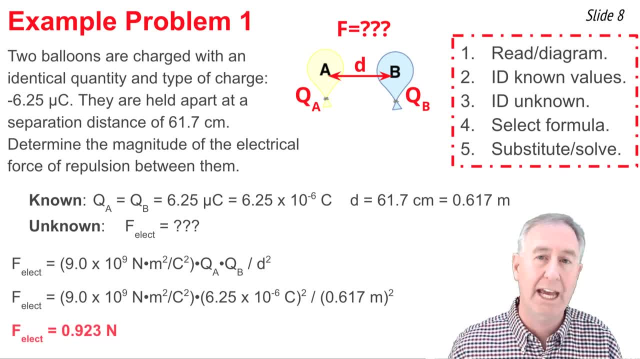 that I know how to use And I carry out the completion of this problem on my calculator Carefully. I enter numbers in the proper operations and I get .923 Newtons as my value for AF electrical. In Example Problem 2 I have two balloons. 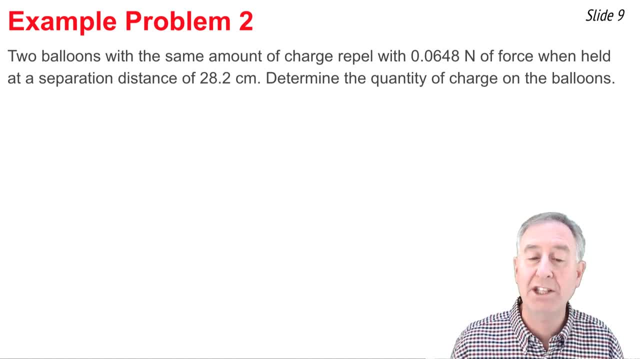 with the same amount of charge. And I know the force of repulsion between them- .0648 Newtons. This occurs when they're twenty eight point two centimeters apart. so my mental picture is that I have two王s and I know the force of repulsion between them- .0648 Newtons- And this occurs when they're twenty eight point two centimeters apart. So my mental picture is that I have two. 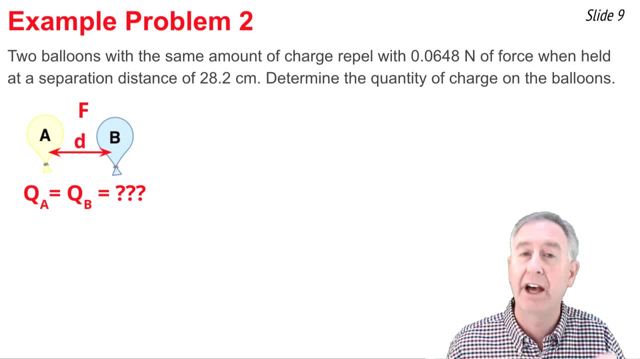 point eight minus. orders are 26 locars per meter against the pressure of fast production and one Falwell. aliens are forces between them with low trials. I've completed this equation is that I have two balloons, I know the force, I know the distance and I know that Q is equal to. 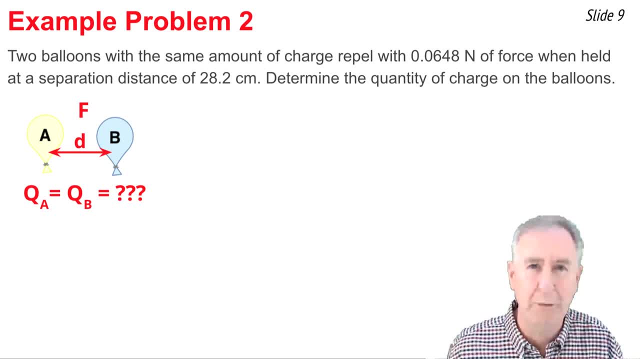 Q. QA is equal to QB, but I don't know what the value is. It's what I'm looking for, So here's what I know. I know F- electrical. I know D- D is given in centimeters and since K value in Coulomb's. 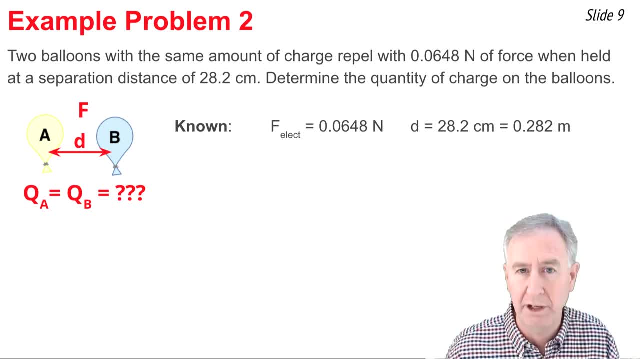 law has meters in it. it's important to divide by 100 and get the D in units of meters. I'm looking for QA and QB Now. here's my equation and it's great for solving for F electrical, but I want to. 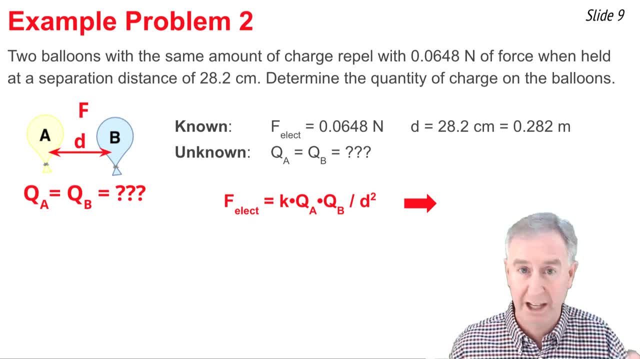 solve for Q. So I'm going to do some algebra Two steps. It goes like this: I'm going to multiply both sides of the equation by D squared to get the D squared out of the denominator on the right side. Then I'm going to divide both sides of the equation by K. That will isolate QA and QB by. 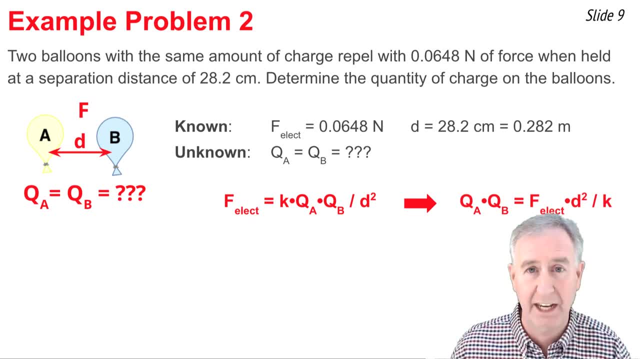 itself on one side of the equation and it looks like that: Now I'm looking to solve QA and QB by D. Now I'm looking to solve QA and QB by D. Now I'm looking to solve QA and QB by D for q a and q b. so here's the equation. but since they're the same q, i'm just going to call them q. 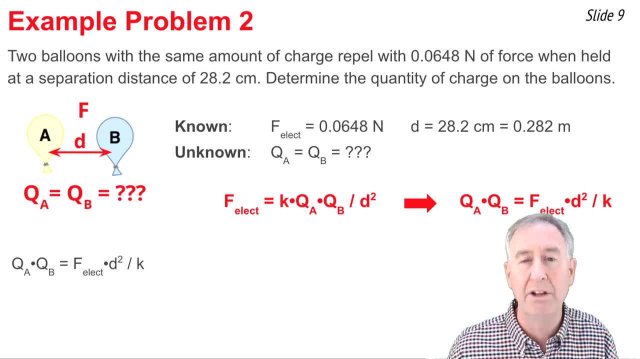 in other words, q squared is equal to f electrical times d squared divided by k. i'm going to now take values of f electrical, of k and d squared and substitute it into this equation. then i'm going to use a calculator i'm comfortable with to find out what q squared is equal to. i'm going to do: 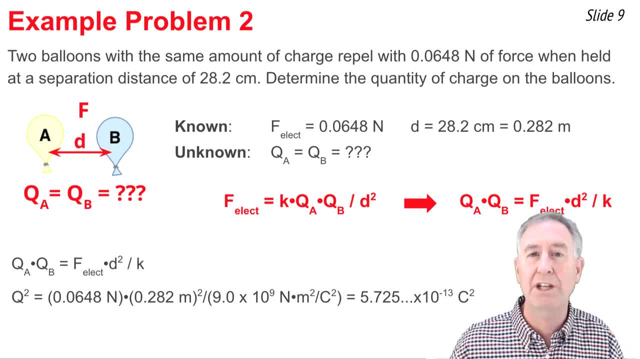 all that mess on my calculator comes out to be 5.725 times 10 to the negative 13th coulomb squared now, that's q squared. i want to solve for q. so if i take the square root of both sides- the left side- 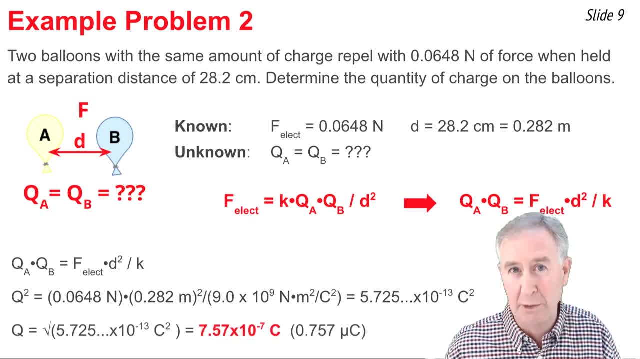 becomes q and the right side becomes the square root of 5.725 times 10 to the negative 13th. do that square root on your calculator. you get 7.57 times 10 to the negative 7th coulombs for the value. 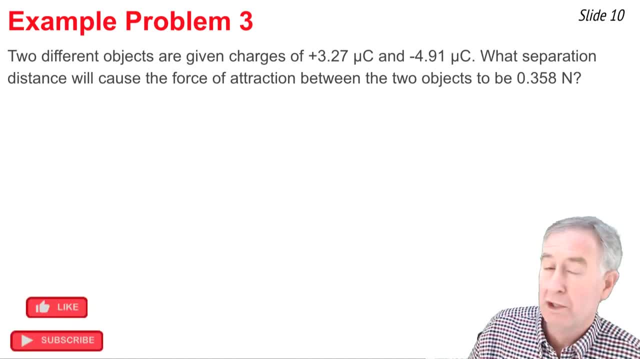 of q in example. problem three: i know the values of qa and qb. they're stated for me and i know the force that acts between these two charges. i'm looking to calculate the separation distance between these two charges. so my mental picture is: i have two objects, maybe balloons. i know their q values. 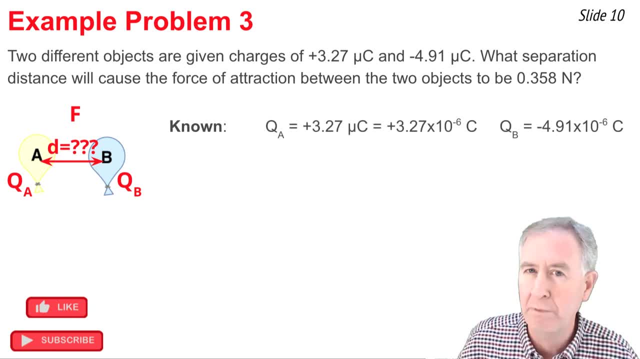 i know the f. i'm looking to calculate the d. here's my known values. i know qa- it's given in micro coulombs- and qb- also in micro coulombs. i want to get it to coulombs, so i'm going to divide these. 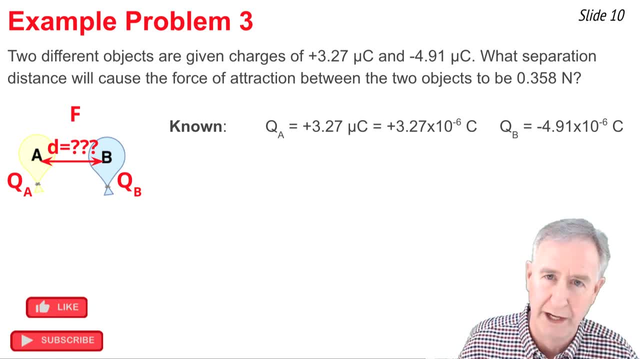 coulomb values: by 10 to the 6th to get the coulomb value. i also know the force. notice how i write those down. now i'm looking to calculate the d, the separation distance, and here's my formula. now the formula is pretty good for solving for f- electrical, but as written it's not real good for solving for d. 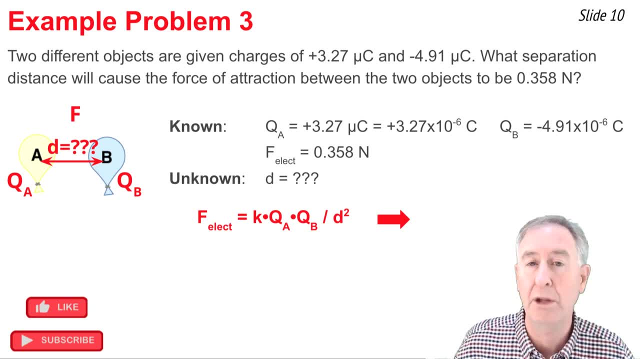 so two steps of algebra. the first step is i'm going to multiply both sides of the equation by d squared. that gets d squared. out of the denominator it would show up on the left as d squared squared times F- electrical. Then I divide both sides of the equation by F- electrical. That gets 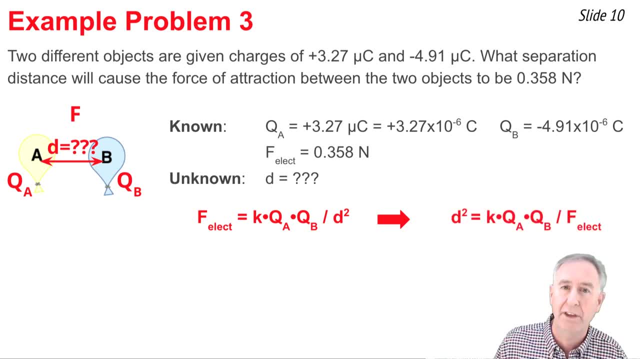 D squared isolated by itself, and here's the result. Now I'm solving for D, so I really would like to take the square root of both sides of this equation. The square root of D squared is D, and that would be equal to the square root of all that other stuff. Now I'm going to take values of.